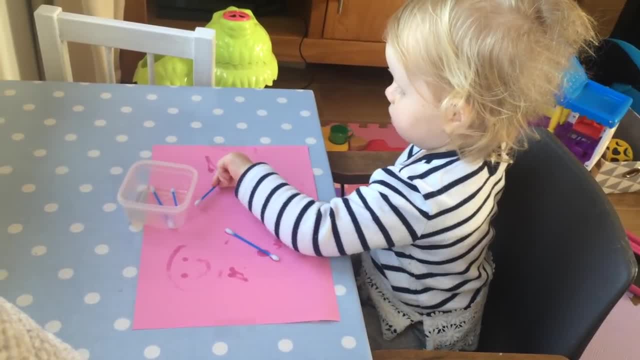 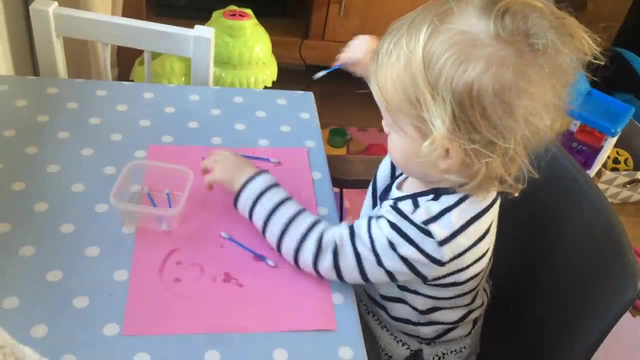 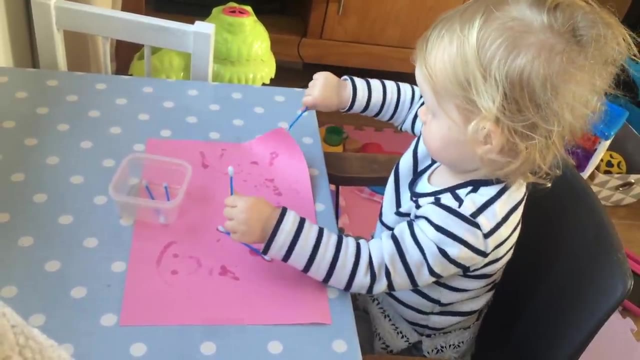 herself. I've used the cotton buds because they're a little bit finer than a paintbrush and it just means that if she was to use a paintbrush the paper would be covered really quickly. so by giving her a little fine implement like a cotton bud, then she can play a little bit longer. Elle really enjoyed this. 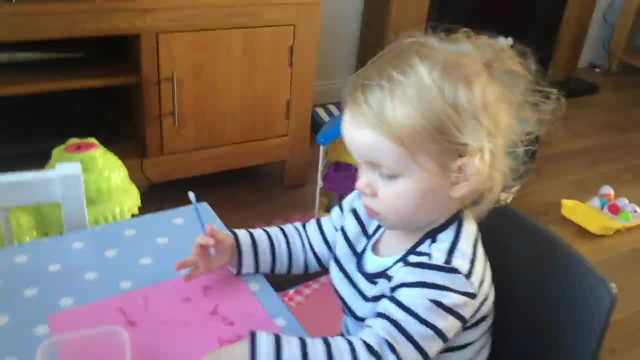 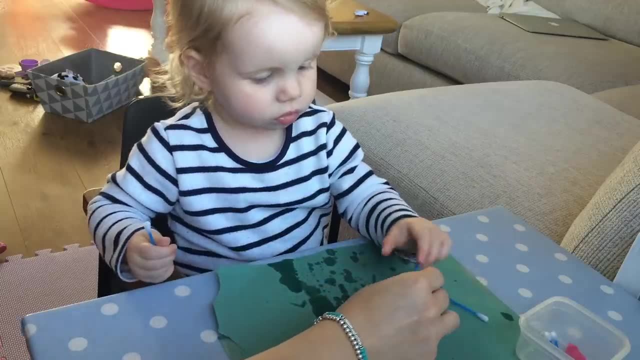 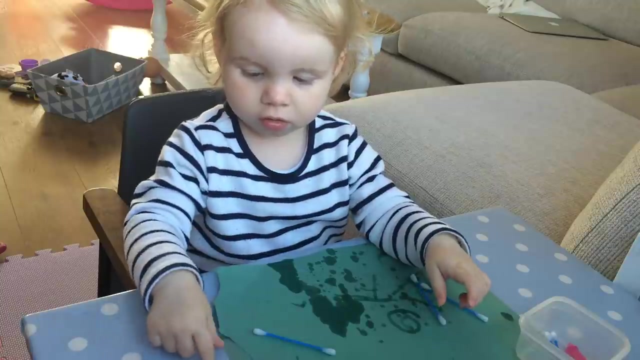 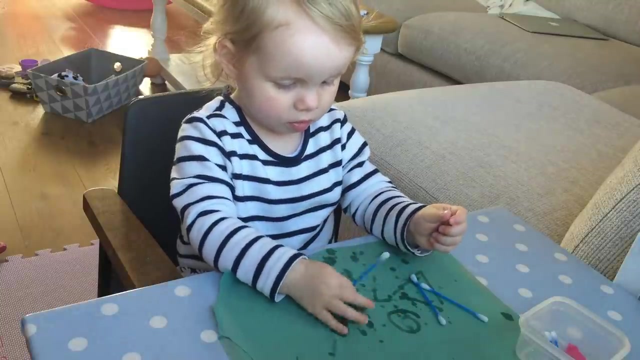 activity and she played with it for quite a long time. Once the paper got too wet and it got a bit torn, we moved on to another colour of paper. Uh yeah, Good girl, This activity is great for encouraging your child to find motor skills. 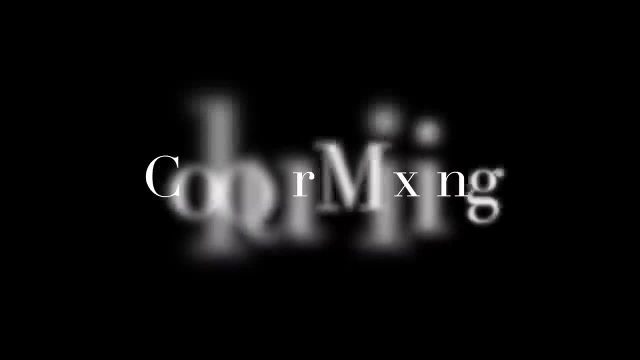 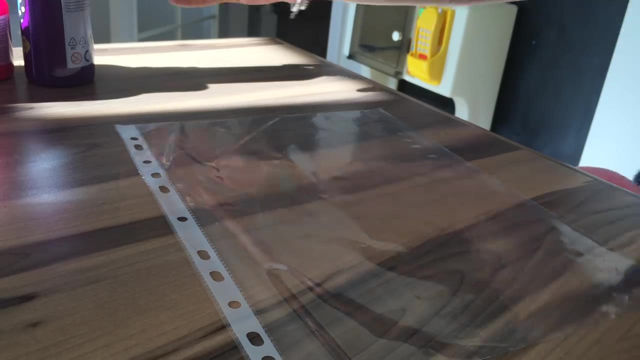 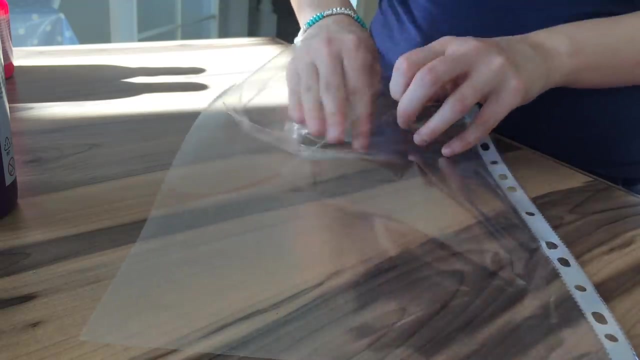 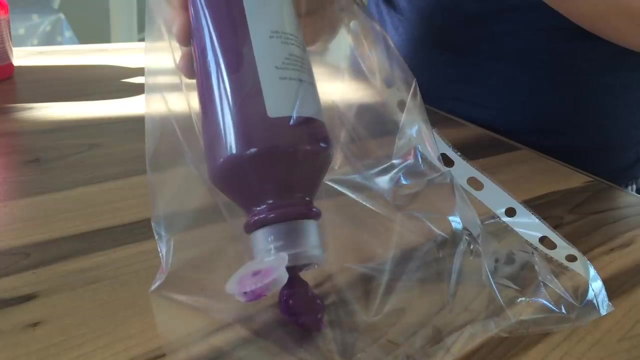 so for this activity you need a clear poly pocket, the kind that you get in ring binders for storing bits of paper, one of those we have loads lying about the house. hopefully you do too. if not, you can pick them up in stationary shops. then you just need to get some paint. 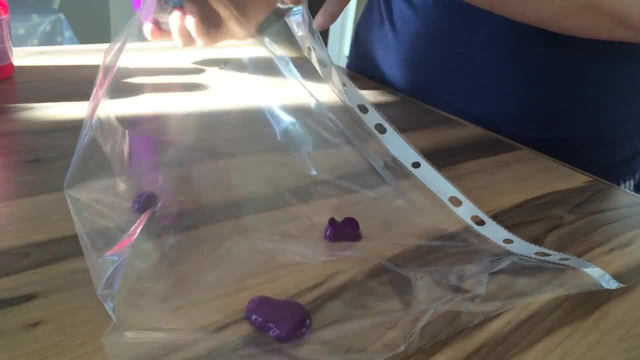 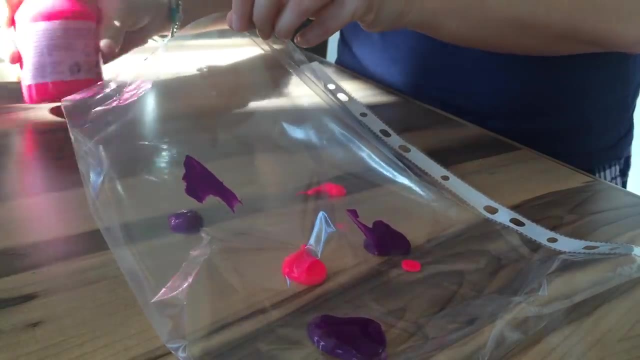 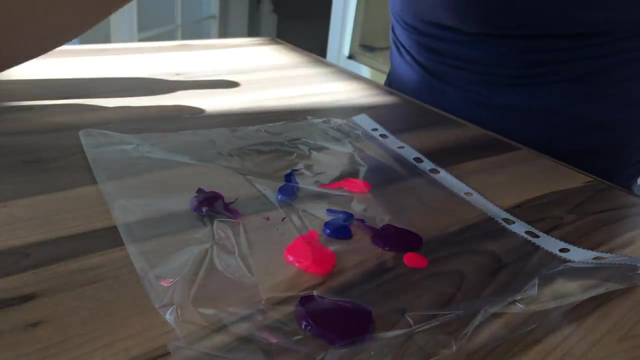 i've got some purple here. just do a few splodges inside the bag and a little bit of pink. i just got the tesco's own brand, kids craft paint. i've added another a bit of blue here. you can use whatever colors you like, and then what you want to do is take the open end of your poly pocket and fold it over like: 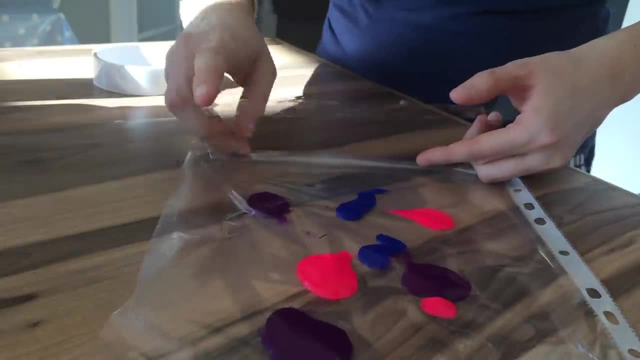 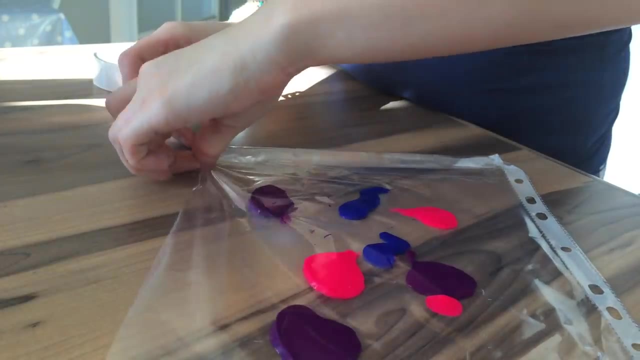 i'm doing here: i fold it over a couple of times just to make sure it's really secure and then add some sellotape to close it shut. and i folded it around the edges just to make sure it's really secure and you get no paint. 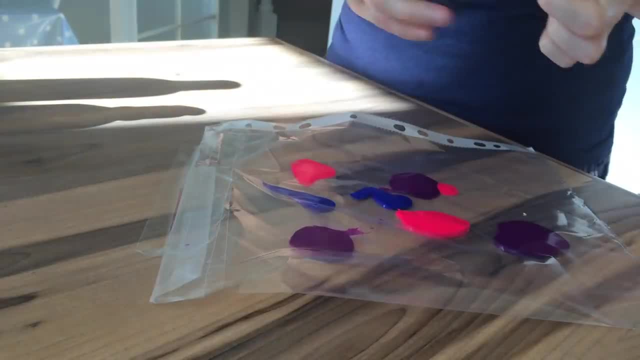 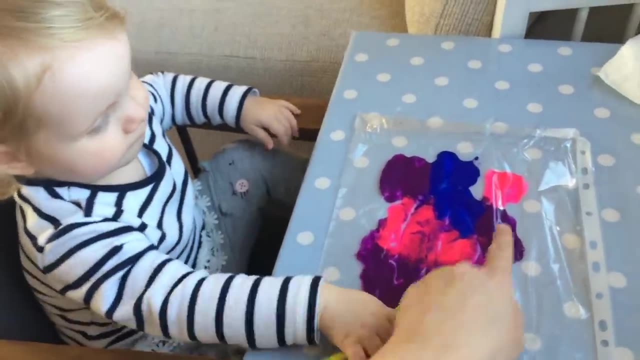 you can then fold it around the edges just to make sure it's really secure and you get no paint leaking leakage. then i've had a little bit of tape to each side of the file just so that i can stick it down to the table that elle's going to be working at. and there we go, i stuck it down to the table and i'm 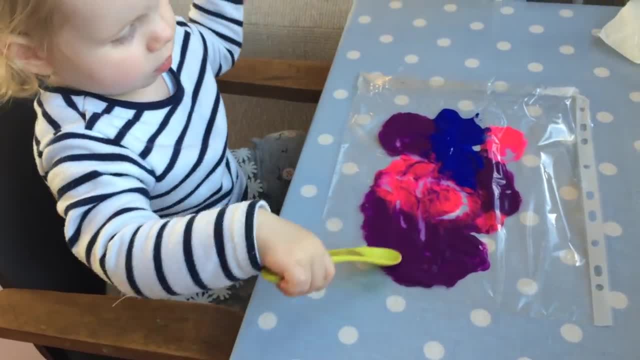 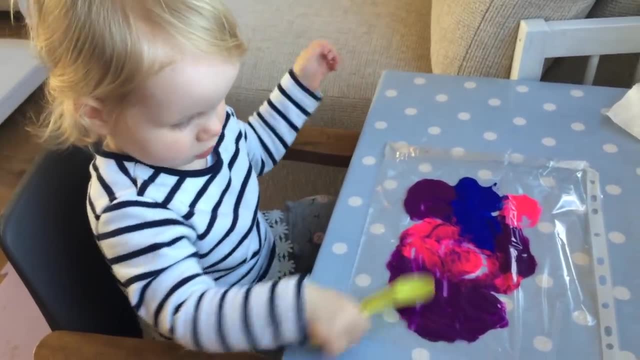 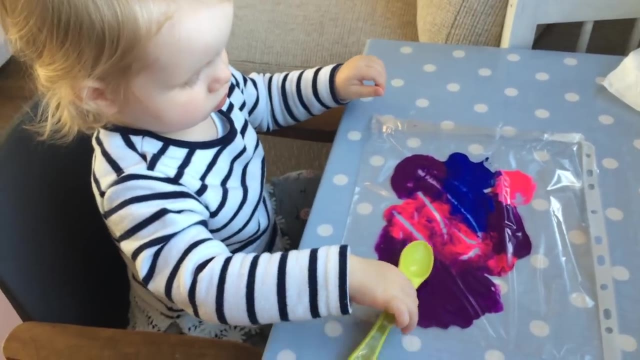 just showing el how to mix the paint using our fingers. i've also given her a spoon to make it a little bit easier for her, and then she can use that to make markings in the paint as well. mix it, oh look. el also took out one of the cotton buds that we've been using earlier and used that to make some markings as well. 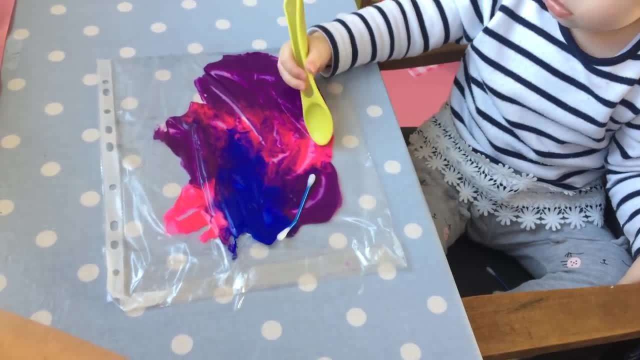 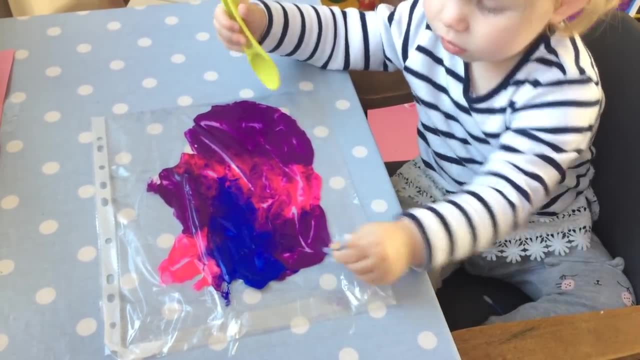 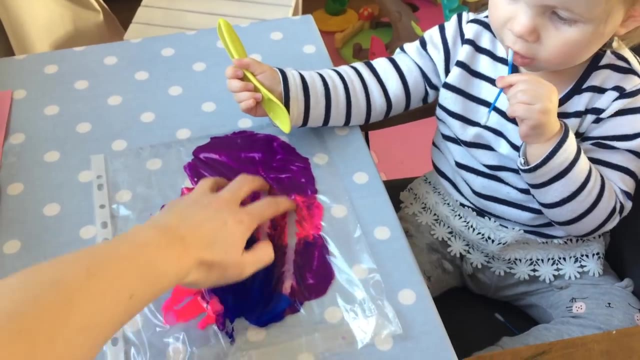 this probably wasn't one of el's favorite activities of the activities that we did for this video, but all children are different. it didn't happen to be el's favorite, but it might be your child's favorite. it'll help them with their manual dexterity, holding on to implements and using their hands. 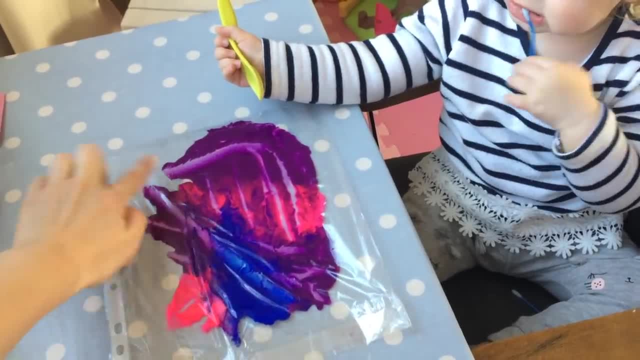 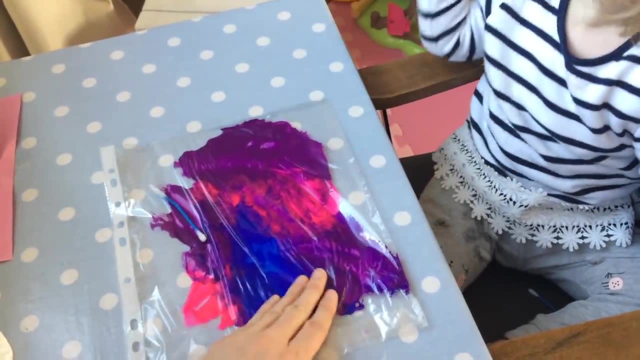 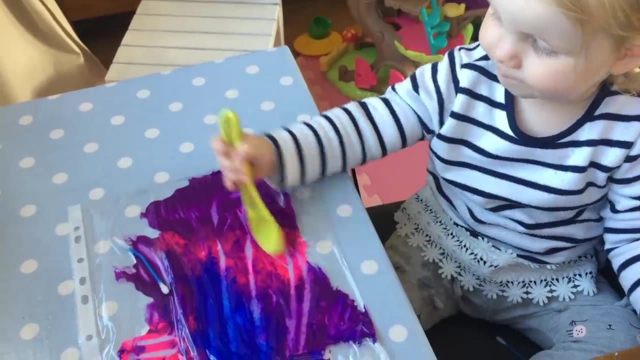 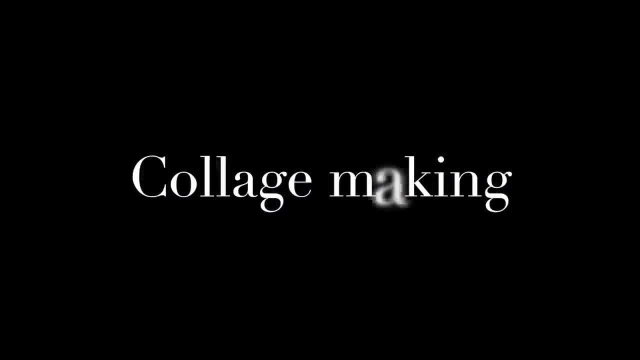 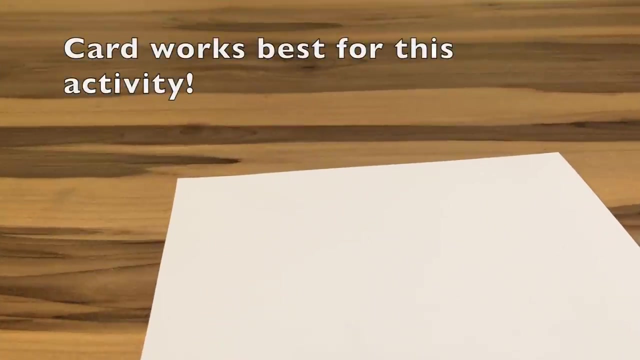 and improve the strength in their hands, which helps for when it comes time for them to be writing cool, look pretty. so the next activity we did later. so the next activity we did later on the evening, after Elle got out of her bath and I just took a piece of white card. It's easier to. 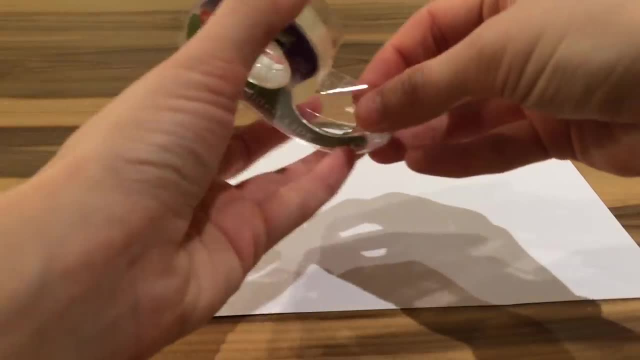 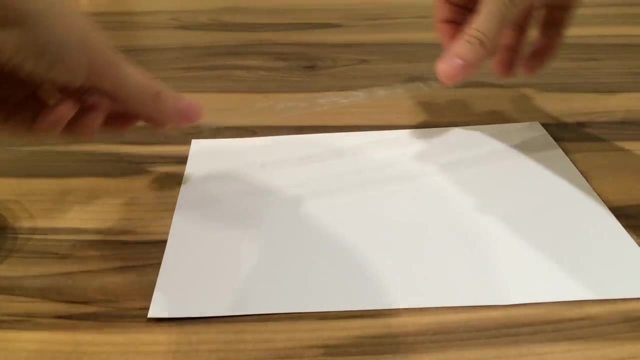 use card than paper for this activity and I got some double sided tape. It only cost me £1.25 from my post office and you can pick it up in supermarkets and other stationary shops and things. It's not very expensive and all I did was take some of the double. 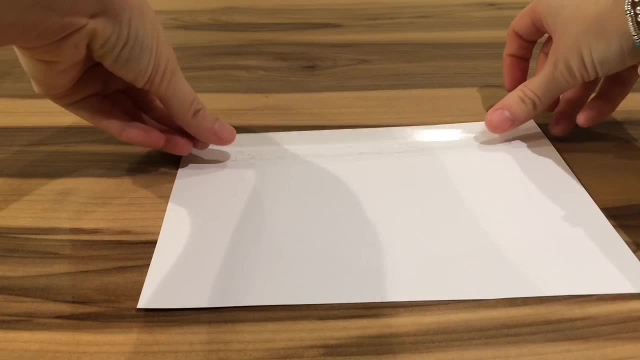 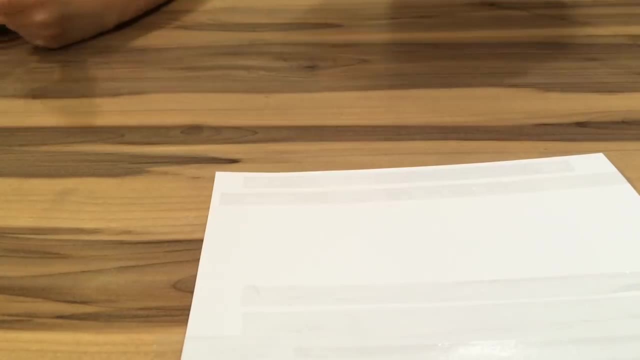 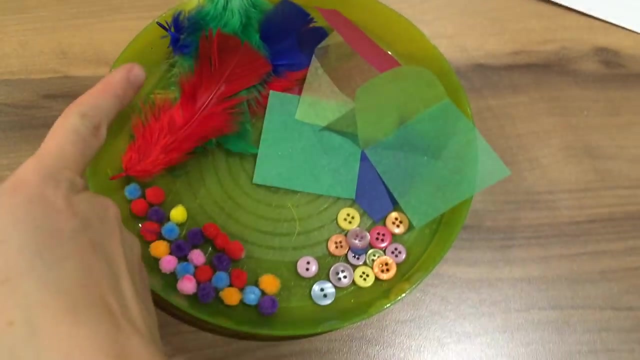 sided tape and start sticking it down across the piece of card. I just continued to do that until I'd covered the whole piece of card with double sided tape. Then I put out a selection of items for sticking and gluing. Here I've got some feathers, some mini pom. 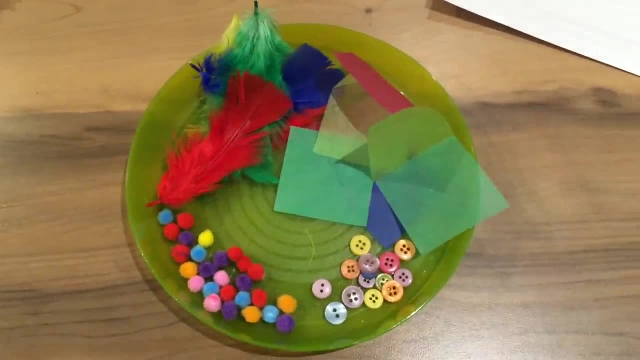 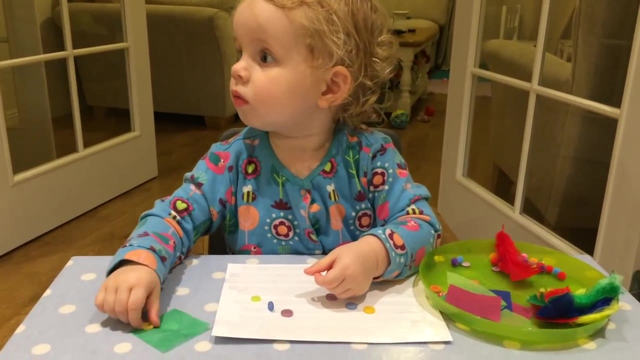 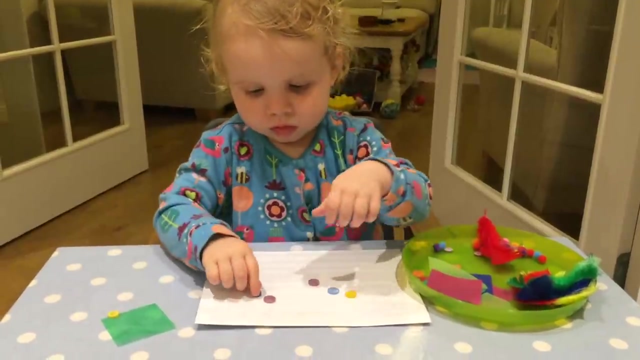 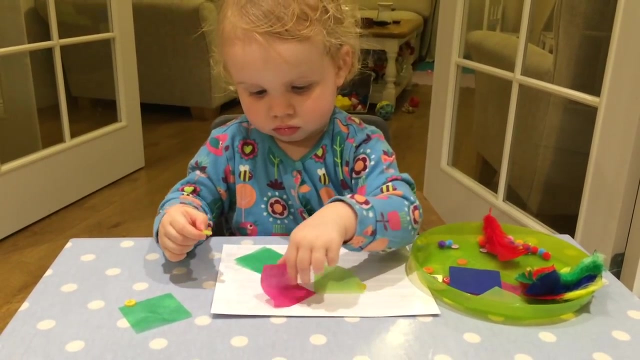 poms, some buttons and some cut up pieces of tissue paper, And then I left it to Elle to make her masterpiece Again. this is really good for encouraging their fine motor skills: Picking up the tiny items like the buttons and the tiny pom poms.